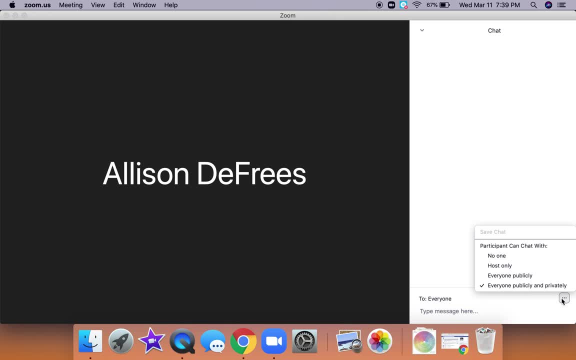 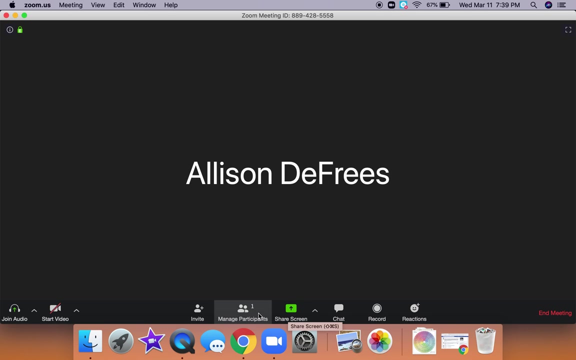 appear on the side here and you can send a message to everyone, or you can change that and you can send a message to a certain student. You can also share announcements or things like that through the chat box if you want to. It's easy to close it out up here by clicking that button. I'll come back to share screen in a minute. You can manage your participants here. You can see everyone who's here. You see that I'm present. 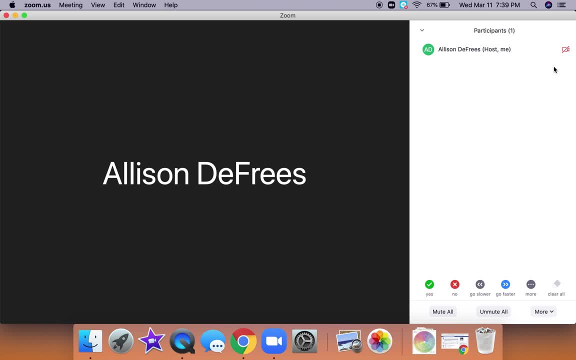 and my red camera has a line through it. That means my cameras turned off And these are buttons that your participants can use. Here are some more buttons: Thumbs up, Thumbs down, Clapping. These would be some buttons you could use with your class if you were. 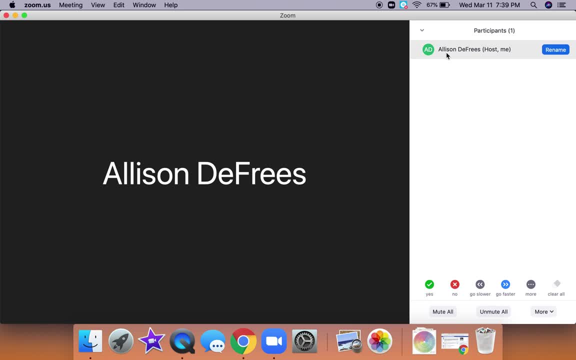 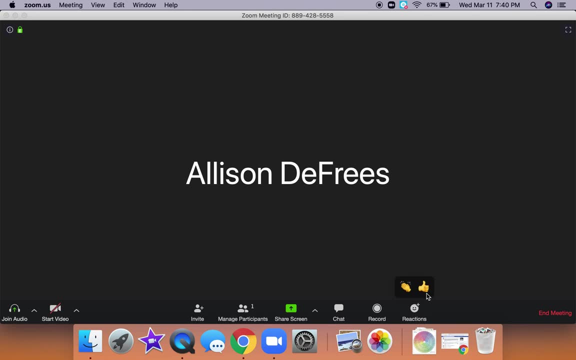 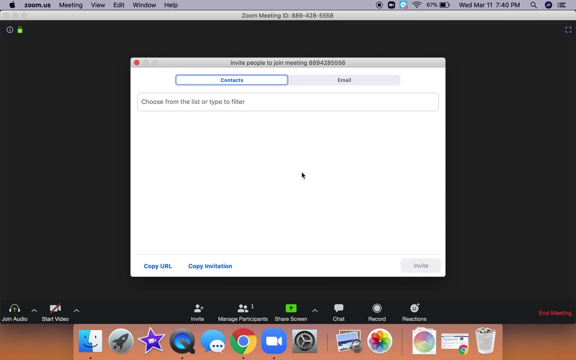 meeting with them. I haven't explored a lot of those buttons because I tutor students individually through Zoom, so I don't get into that a lot, Although we love the reactions. We love the things that happen as a student. thumbs up Okay And the invite button is pretty self-explanatory. You can invite people to your. 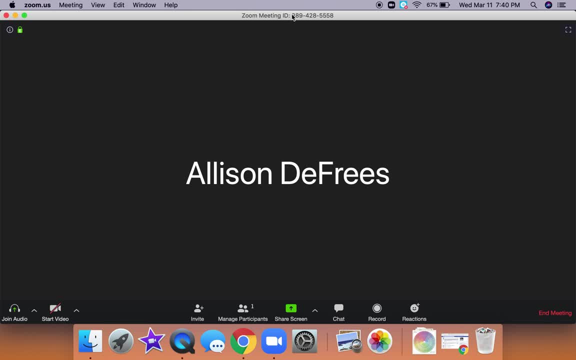 meeting. Okay. Another basic thing about Zoom is at the very top you have a meeting ID. It's in the top bar, the gray bar, here at the top. It'll pop up. There it is. It's a long number and a. 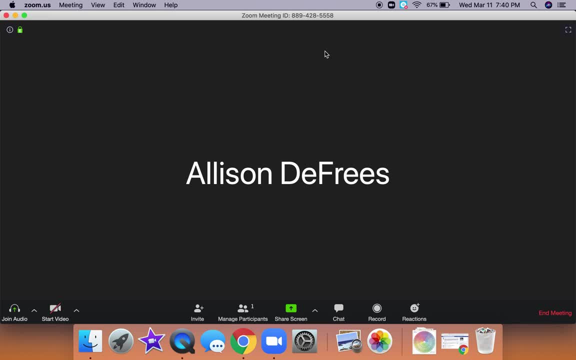 10 digit number And that's the meeting ID that you would share. It's just like a conference call where you have to type in the number to join the call You can put. you can make that a special number, or Zoom can auto-generate just your basic conference room and give you a number. So I can. 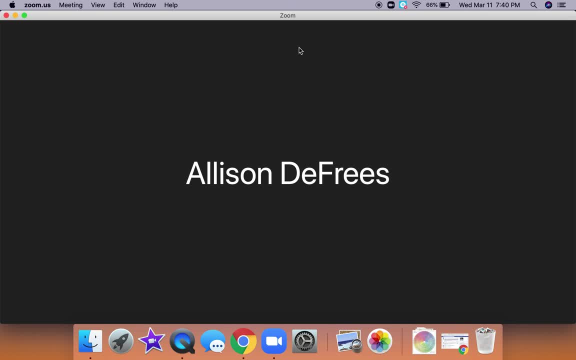 imagine teachers wanting to send that number to their parents or post it on their private classroom site, a private Facebook page, and say: join me on Zoom at 1 pm. And here's the the um Zoom meeting ID code. It would be like typing in the code to join Kahoot. It'd be very similar. 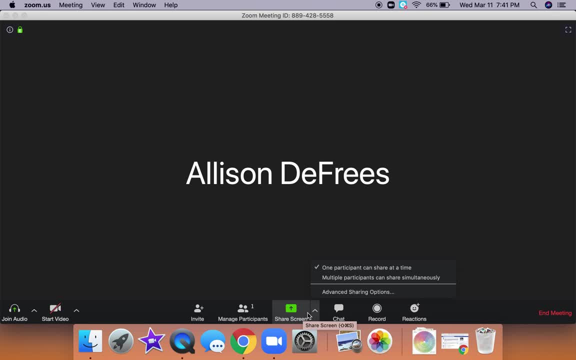 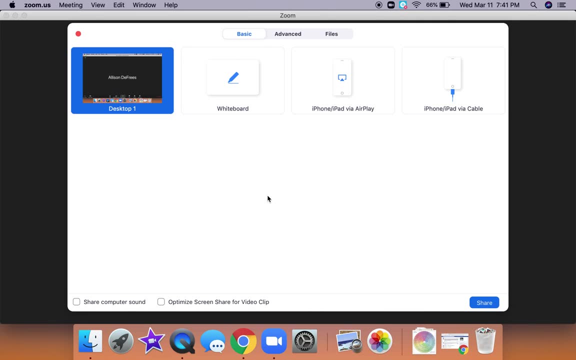 Now I'm going to share my screen with you. Um, you can also ask your students to share their screen if you wanted, if you said, okay, well, um, you know, this one student has the correct answer on their math problem. I want to see their.